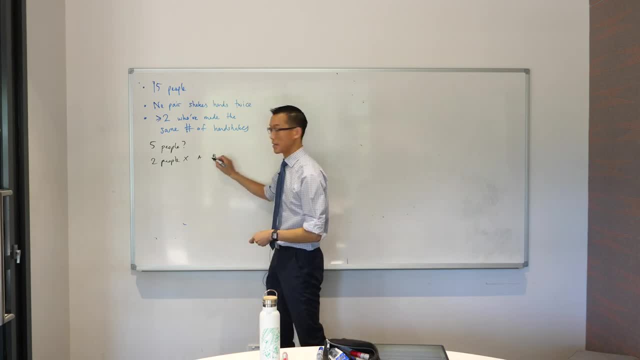 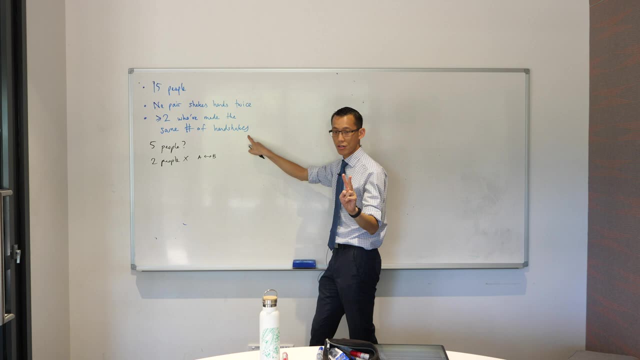 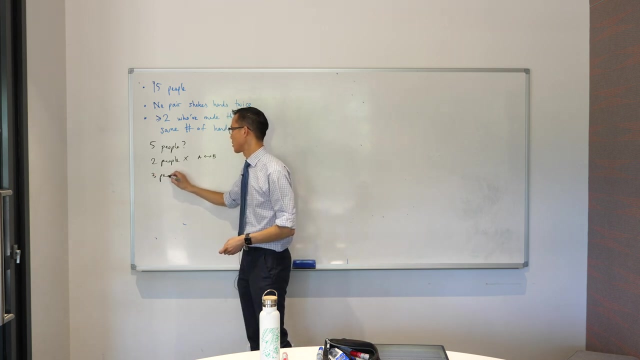 people come in A and B, they shake hands, that's it. there's no more shaking that can happen, because no pair shakes hands twice. Is this true? And the answer is yes, the two people are the only ones there. Let's think about three for a second. 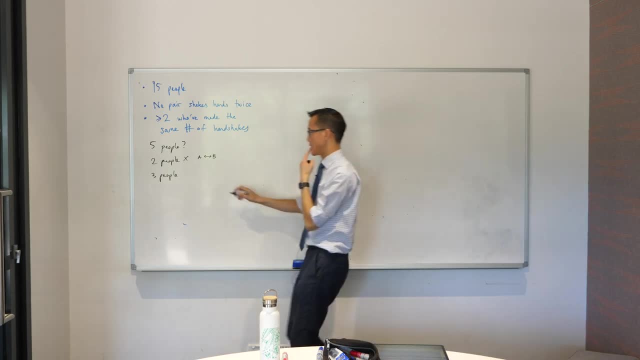 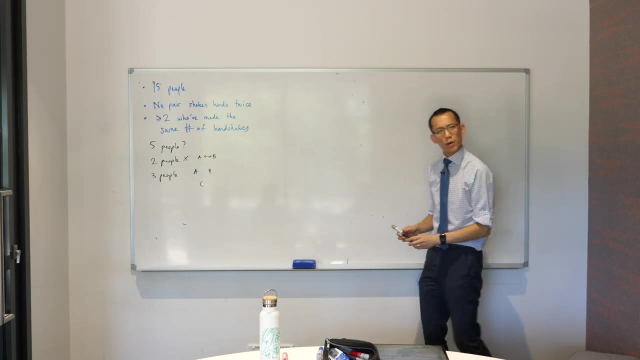 Hmm, think about it for a moment. So now I've got A, B and C right, I'm going to get to our case of five in a second, but I want to build my way there. okay, What could happen? 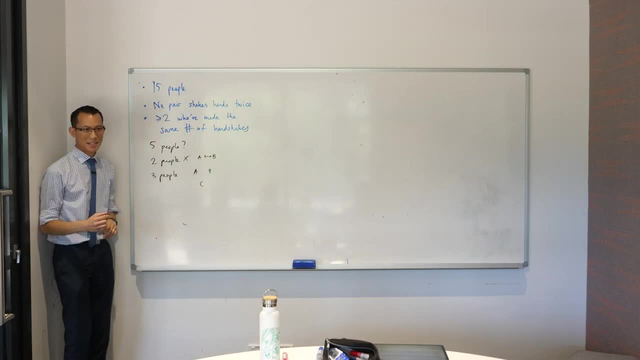 Well, for starters, actually nothing could happen, right? I mean, I know they said people start shaking hands, but in this situation right now, is the statement that they've suggested to us? is it true? The answer is yes, right, Because so far all three people have never shaken hands. 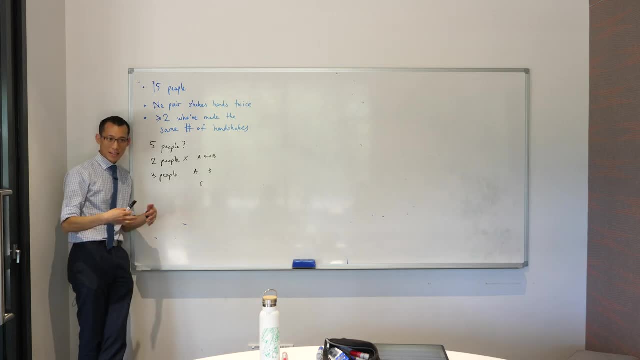 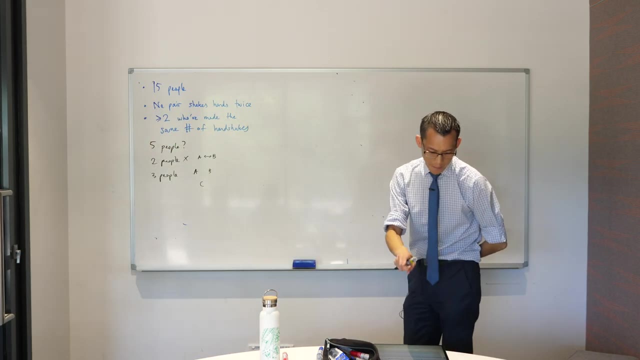 with anyone, so they're all at zero, as it were. okay, But even as I start to think about what happens right at each stage, because if I look back at the question, you look back at it with me as well- many handshakes happen, but we don't know how many, like it's kind. 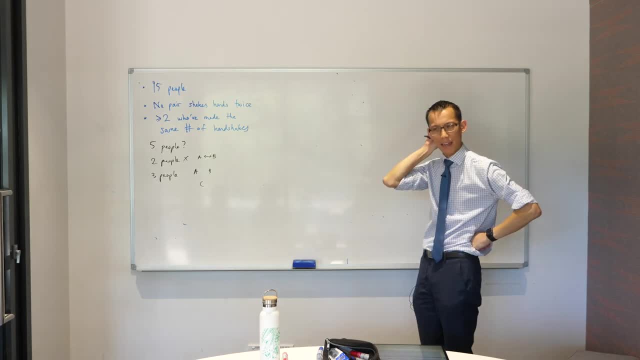 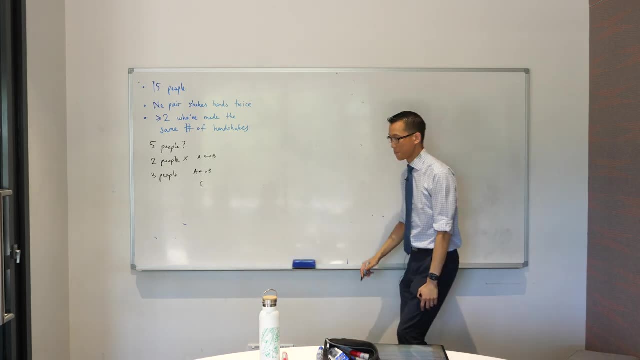 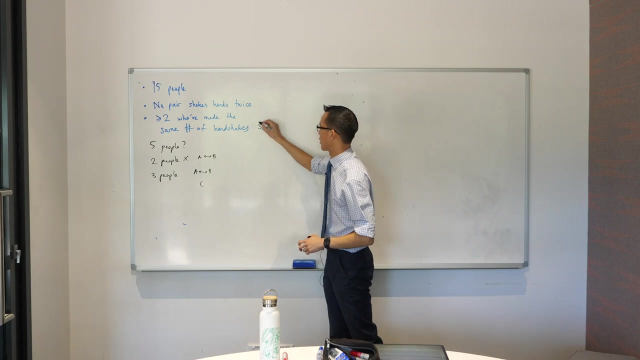 of open, which is part of what makes this problem a bit vague and confusing, right. So what might happen? lots of different things could happen If those first two original people- they shook hands right At this point, right here, does the statement I'm going to call this statement S by the. 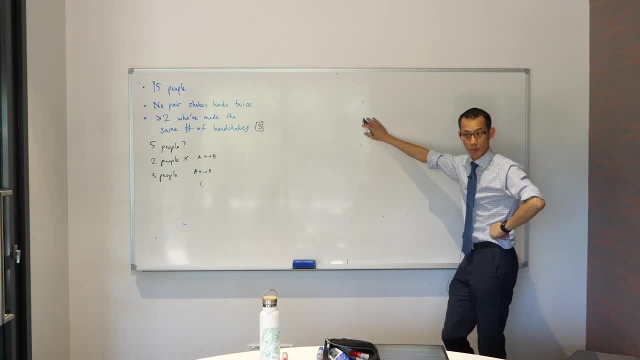 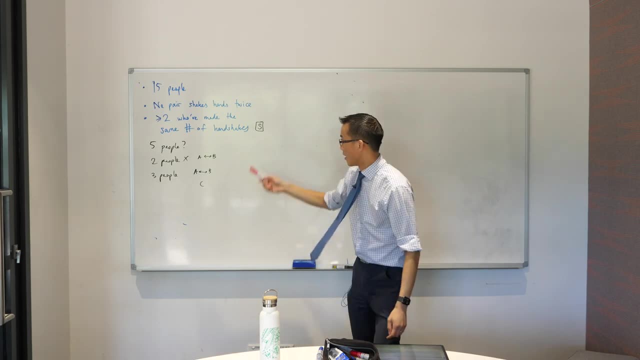 way, just so I can stop saying this statement is S true at this point. It is right- And maybe what you want to do with me, by the way I'm writing- to think This can sound strange. This writing is a way of communicating thinking to you, but 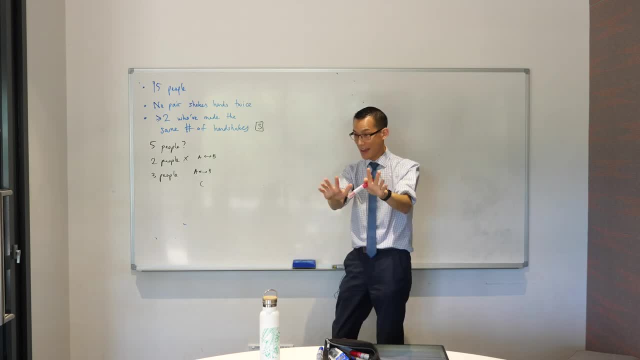 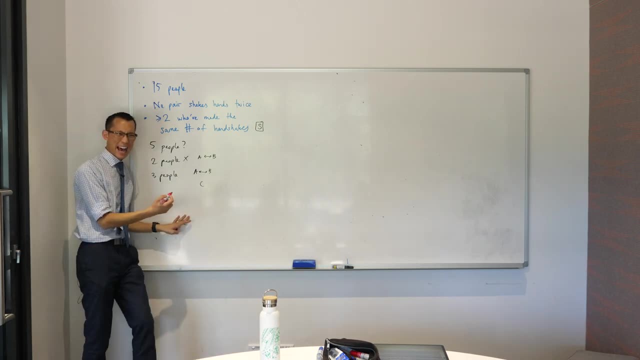 it's also actually my way of constructing my own thinking, So I highly encourage you. Okay, Whatever it is you want to jot down, this is me trying to think through the problem At the moment. I'm just keeping a tally of how many handshakes have happened for each. 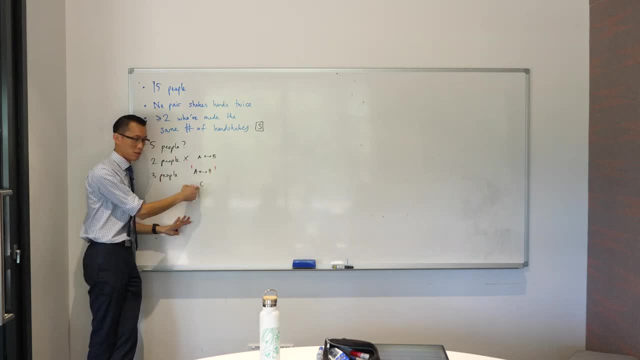 person in this situation. So far, I've got one one and then zero. Yeah, So far, so good. S is still true. Pick another couple of people to shake hands. Who would you like to shake hands? A and C. 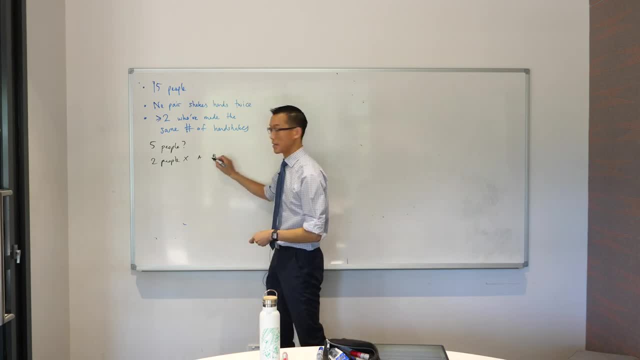 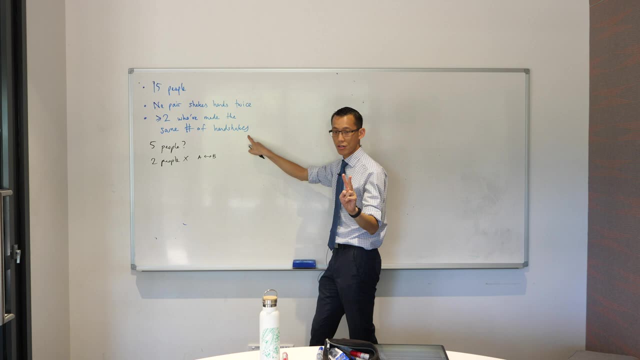 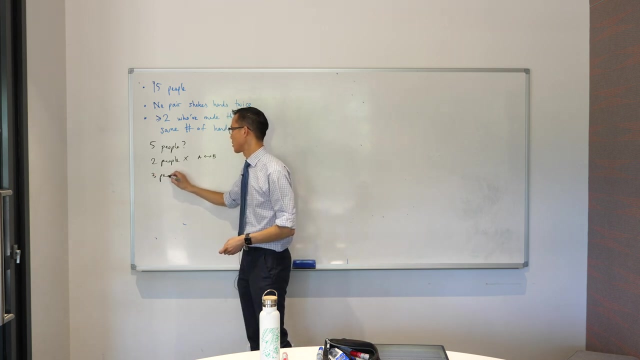 people come in A and B, they shake hands, that's it. there's no more shaking that can happen, because no pair shakes hands twice. Is this true? And the answer is yes, the two people are the only ones there. Let's think about three for a second. 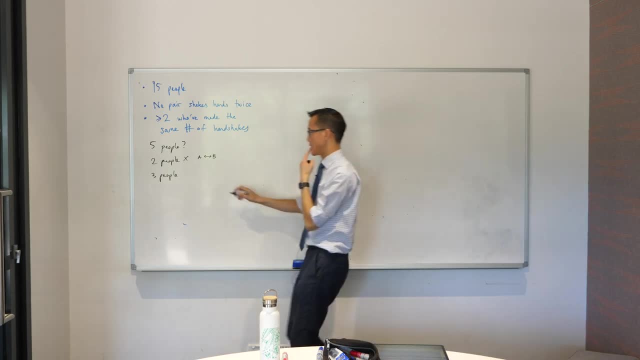 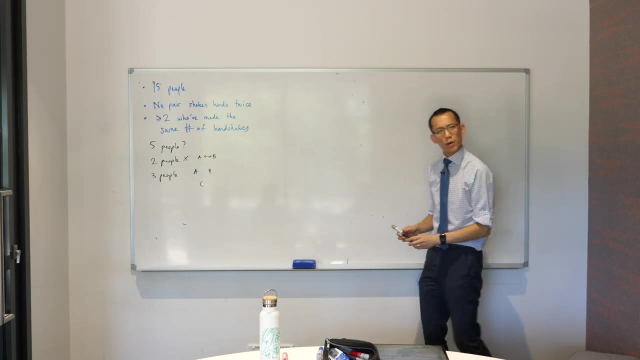 Hmm, think about it for a moment. So now I've got A, B and C right, I'm going to get to our case of five in a second, but I want to build my way there. okay, What could happen? 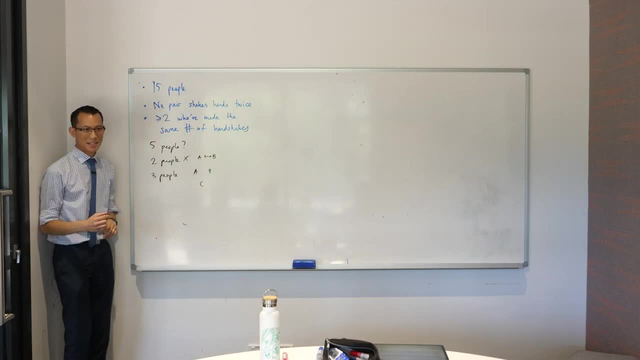 Well, for starters, actually nothing could happen, right? I mean, I know they said people start shaking hands, but in this situation right now, is the statement that they've suggested to us? is it true? The answer is yes, right, Because so far all three people have never shaken hands. 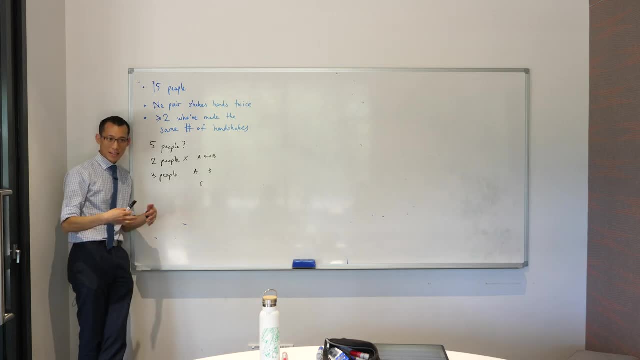 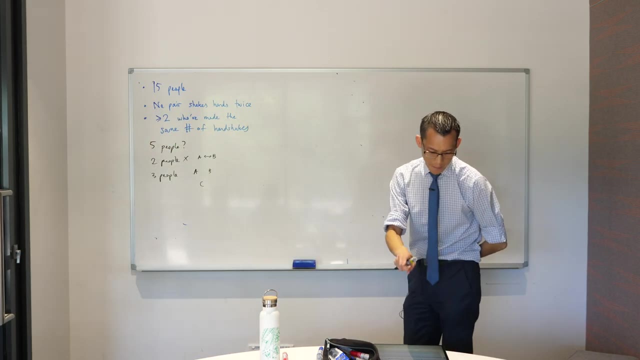 with anyone, so they're all at zero, as it were. okay, But even as I start to think about what happens right at each stage, because if I look back at the question, you look back at it with me as well- many handshakes happen, but we don't know how many, like it's kind. 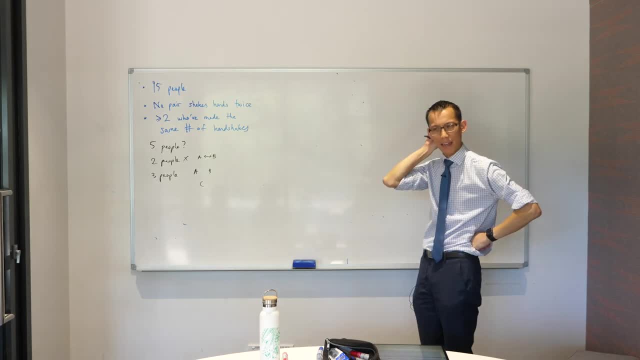 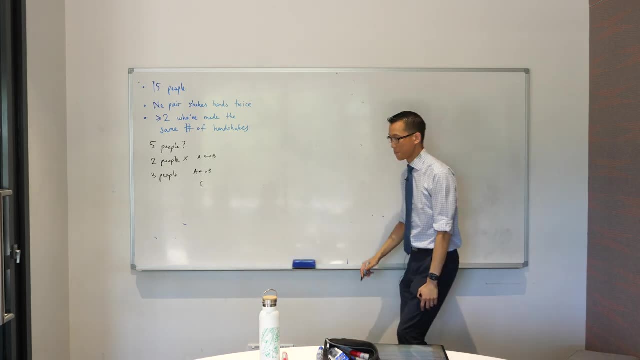 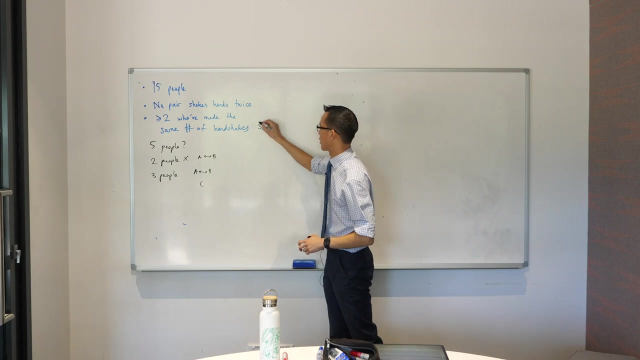 of open, which is part of what makes this problem a bit vague and confusing, right. So what might happen? lots of different things could happen If those first two original people- they shook hands right At this point, right here, does the statement I'm going to call this statement S by the. 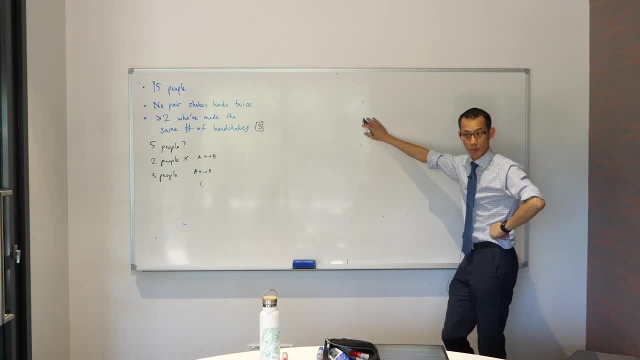 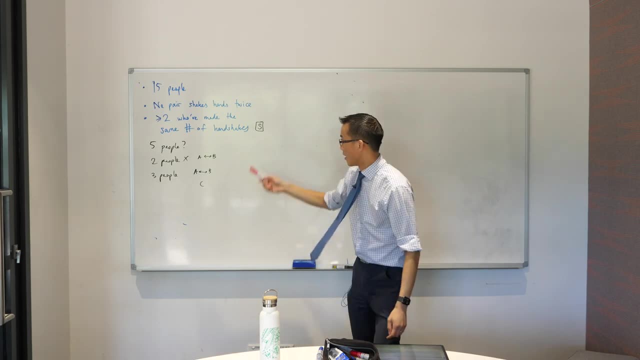 way, just so I can stop saying this statement is S true at this point. It is right- And maybe what you want to do with me, by the way I'm writing- to think This can sound strange. This writing is a way of communicating thinking to you, but 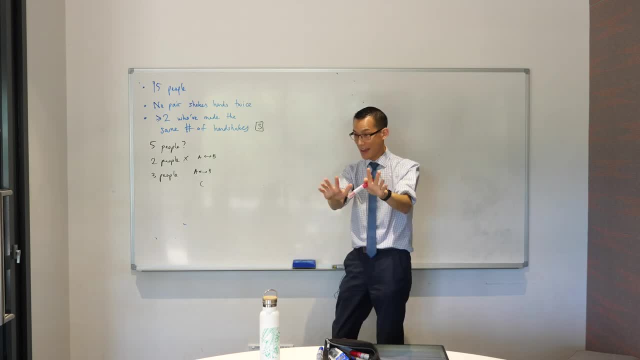 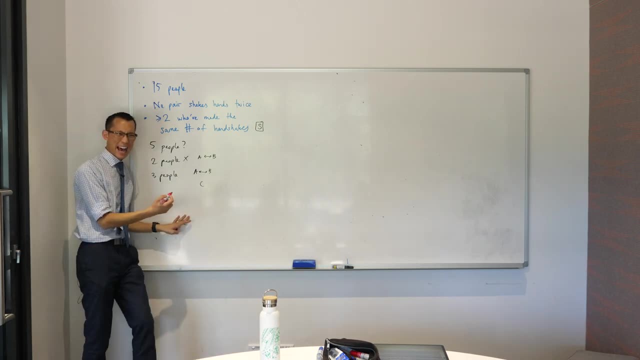 it's also actually my way of constructing my own thinking, So I highly encourage you. Okay, Whatever it is you want to jot down, this is me trying to think through the problem At the moment. I'm just keeping a tally of how many handshakes have happened for each. 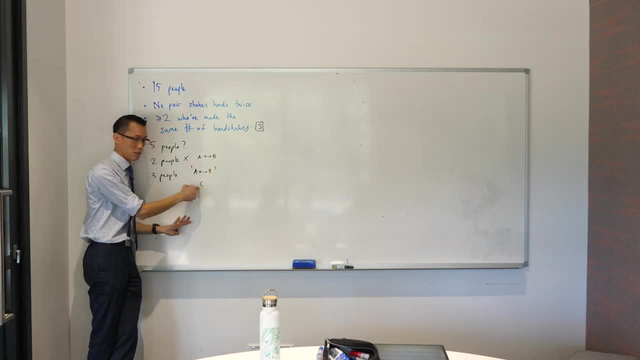 person in this situation. So far, I've got one one and then zero. Yeah, So far, so good. S is still true. Pick another couple of people to shake hands. Who would you like to shake hands? A and C. 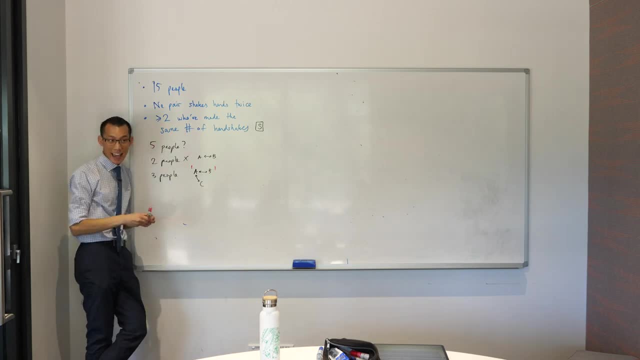 A and C. Okay, So the handshake has happened. This person's up to two handshakes now. Now this person's up to one. So it's all still true. right, S is still true, It's just true with different. 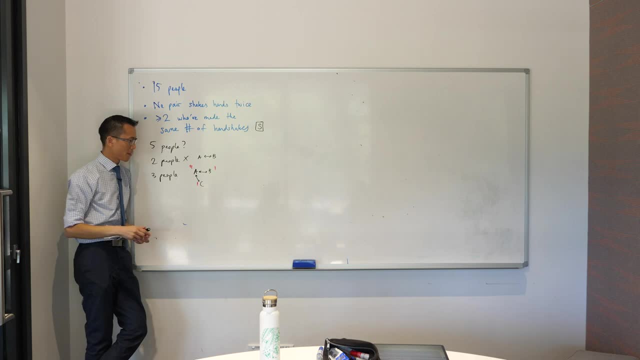 people. Yes, Following Divya. Yeah, I already know it's true at this point, but why not? Why don't we just make them all shake hands with each other? So B and C Now shake hands, And at this point, well, what happens to my tallies? 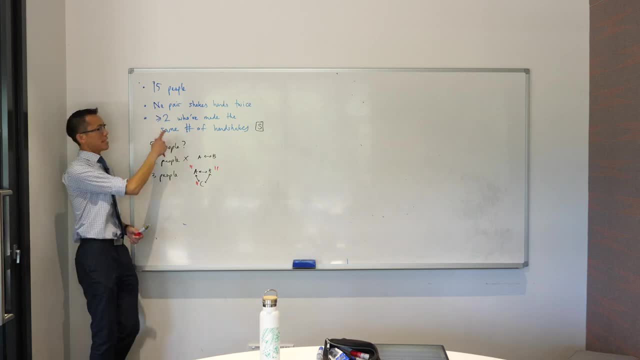 2. 2 and 2.. 2 and 2.. at least two. so the fact that all three of them have done the same number of handshakes is totally fine. Okay, All right, let me pause for a minute. 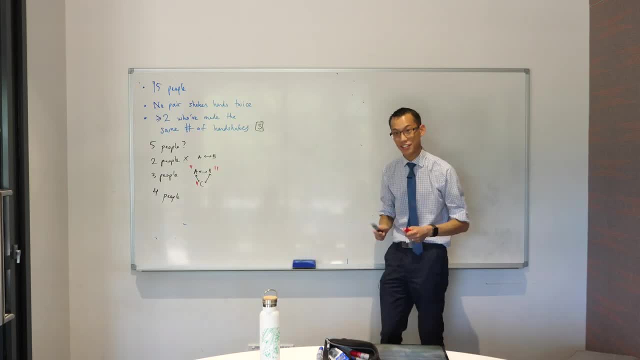 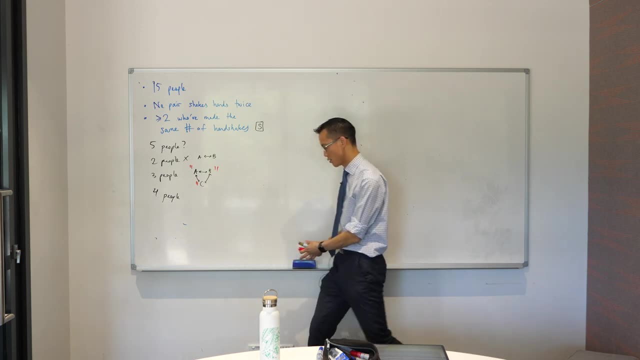 You tell me what happens for four. We're going to get to five in a minute, but I actually wonder if we need to go up to five for you to sense what pattern is forming here. Can I just pause for a minute? I'll actually here you go. here's A, B, C and D. You have a go you model. what's happening? 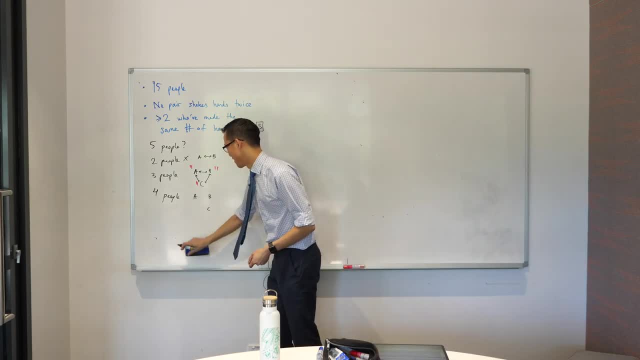 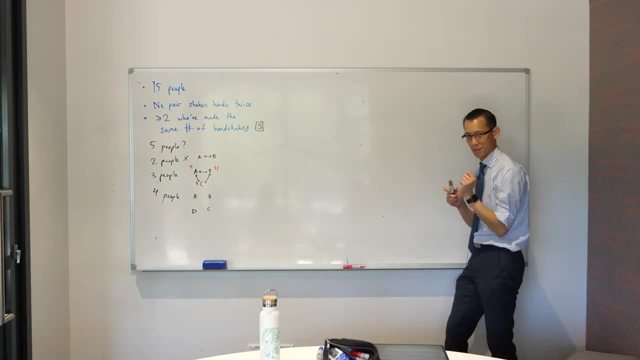 in this situation. I don't know why I drew D so much lower than the rest of them, And then you see, if you can help me reason through what this has to do with the pigeonhole principle, Maybe I should just ask before I let you go. 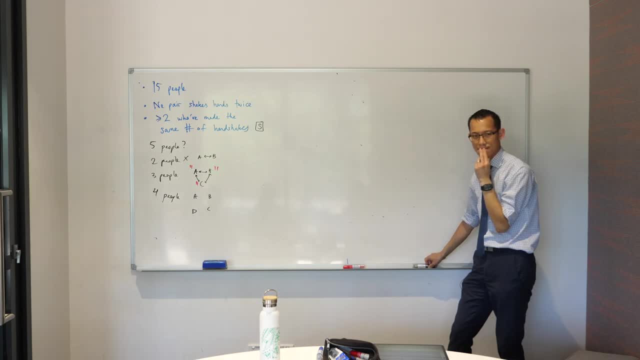 What is the pigeonhole principle again, Can you state it for me? I'll give you a clue. It has to do with pigeons and holes. Do you remember How many pigeons can fit inside a map? Good, So the whole idea is: and it's so strange. 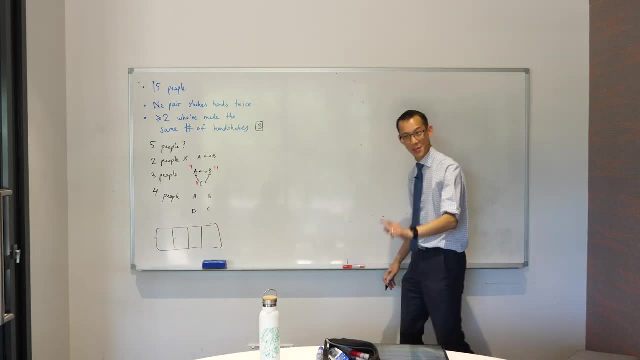 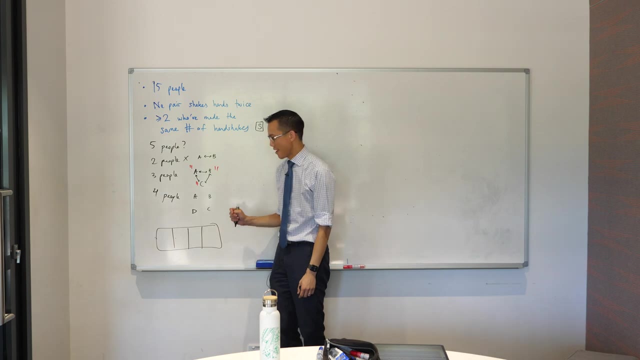 Because none of us deal with pigeons at all and we don't put them in holes. but you can picture it right: If you've got, say, for example, four pigeonholes, right, And you've got five pigeons, okay. 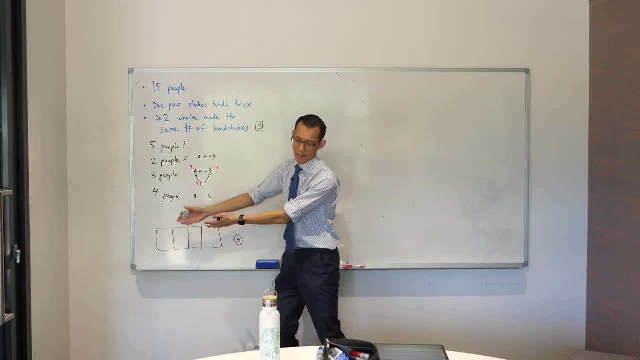 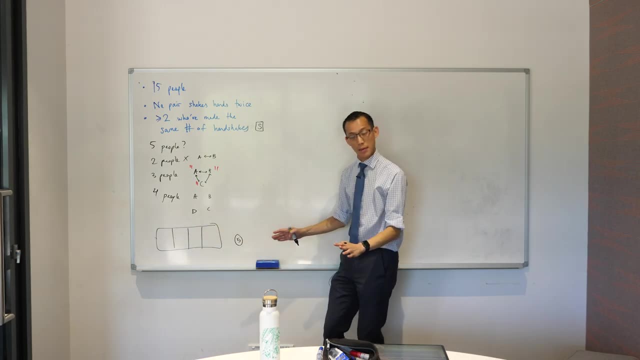 You know that there's going to be- assuming they all go into their pigeonholes, okay, There's going to be at least one pigeonhole where there are two pigeons. There have to be right, Because after you put in one here and then one here, and then one here and then one. 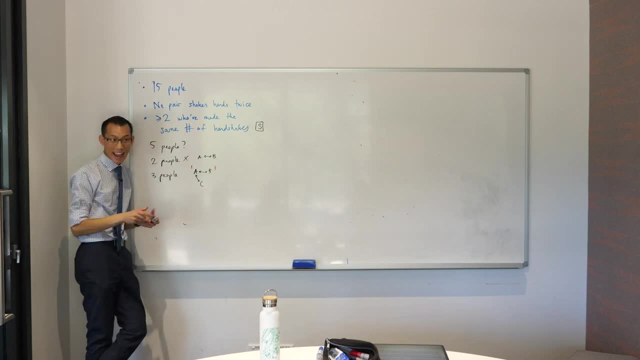 A and C. Okay, Okay, Now that the handshake has happened, this person is up to two handshakes now. Now this person is up to one. So it's all still true, right? S is still true. It's just true with different people. 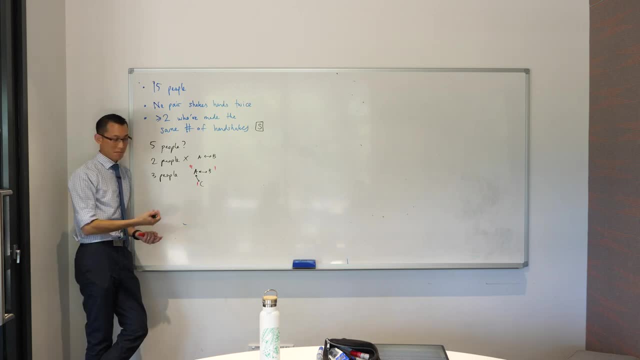 Yes, Following Divya Yep Di. I already know it's true at this point. but why not? Why don't we just make them all shake hands with each other? So B and C now shake hands, And at this point, well, what happens to my tallies? 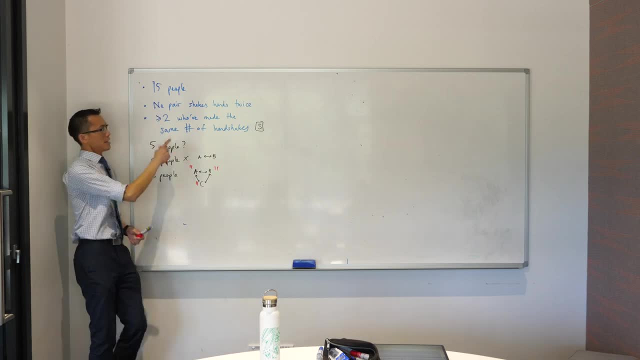 Two and two, Two and two, Two and two least two. so the fact that all three of them have done the same number of handshakes, it's totally fine, okay. all right, let me pause for a minute. you tell me what happens for four. we're gonna get to five in a minute, but I actually 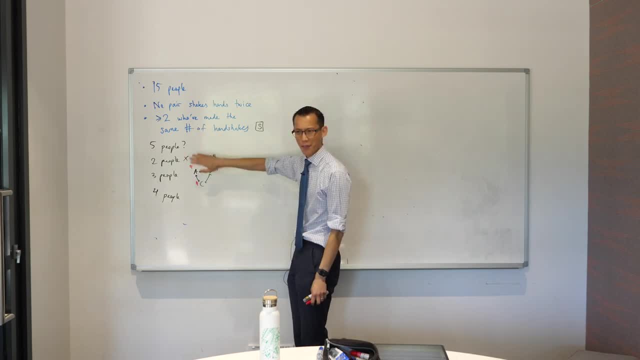 wonder if we need to go up to five for you to sense what pattern is forming here. can I just pause for a minute? I'll actually here you go. here's a, B, C and D. you have a go. you model what's happening in this situation. I don't know. 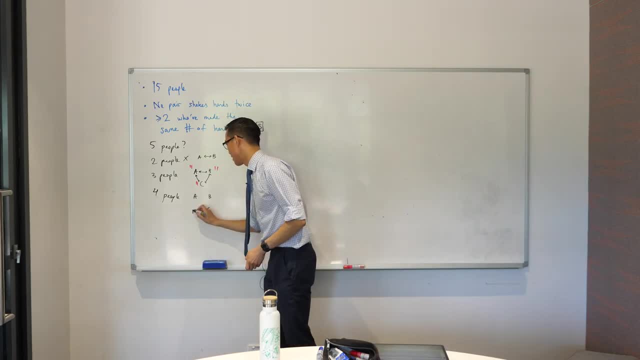 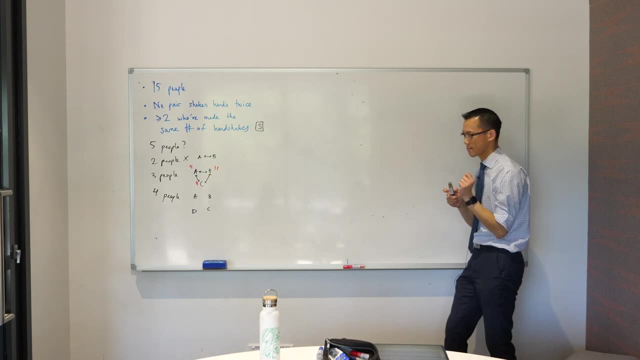 why I drew D so much lower than the rest of them. and then you see, if you can help me reason through what this has to do with the pigeonhole principle, maybe I should just ask before I let you go: what is the pigeonhole principle again, can? 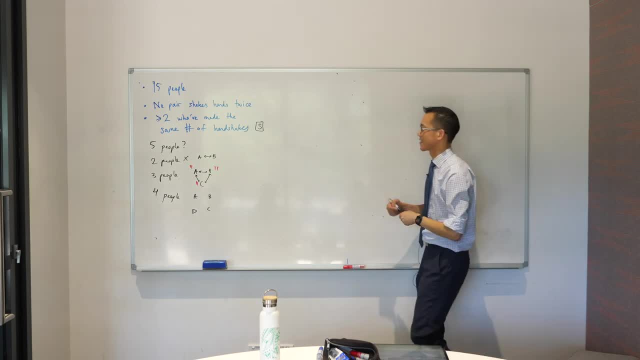 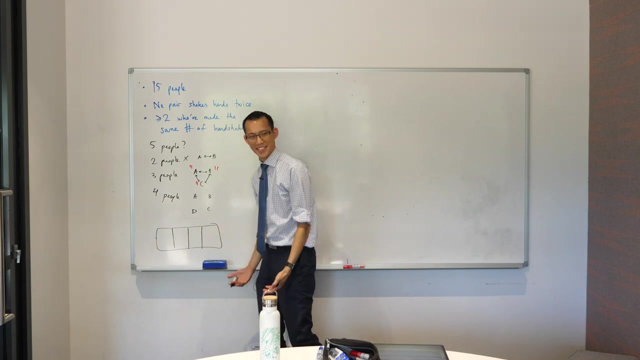 you state it for me. I'll give you a clue. it has to do with pigeons and holes, do you remember, can I good? so the whole idea is, and it's it's so strange because none of us deal with pigeons at all and we don't put them in holes. but you can picture right if you. 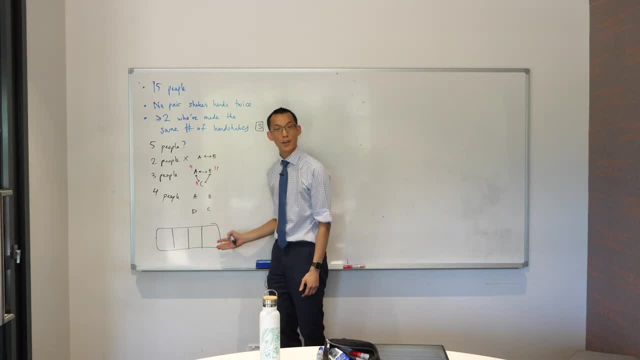 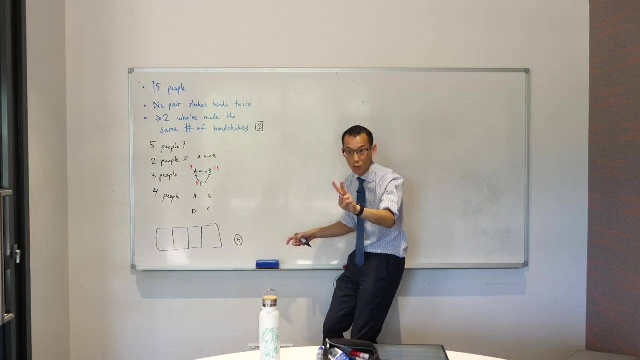 got, say, for example, four pigeonholes, right, and you've got five pigeons. okay, you know that there's gonna be at least- and assuming they all go into their pigeonholes- okay, there's going to be at least one pigeonhole where there are two pigeons. they have to be right because after 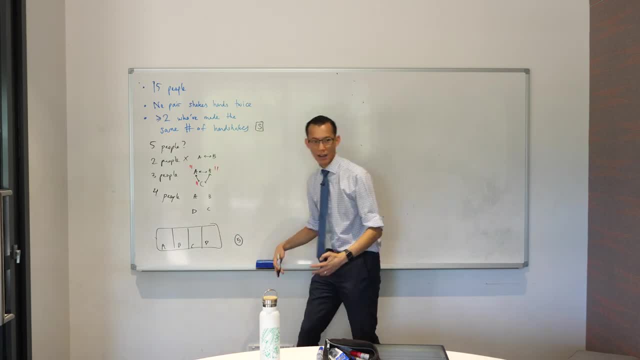 you put in one here and then one here, and then one here and then one here. you're like, oh, I've got my fifth pigeon to put in, but he has to or she has to be in the same pigeon holes. one's already taken. can I say that one more time? and I 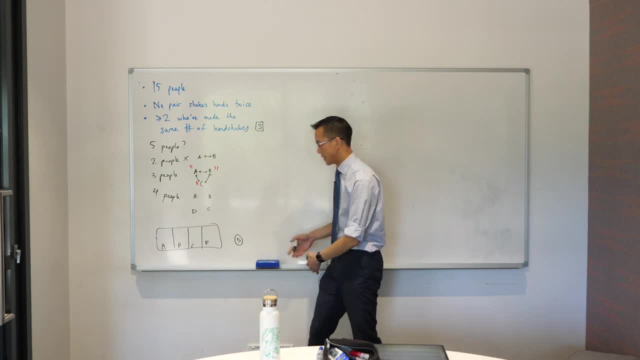 here You're like: uh-oh, I've got my fifth pigeon to put in, but he has to, or she has to be in the same pigeonhole as one that's already taken. Can I say that one more time? And I wonder if you're connecting it to this yet, right? 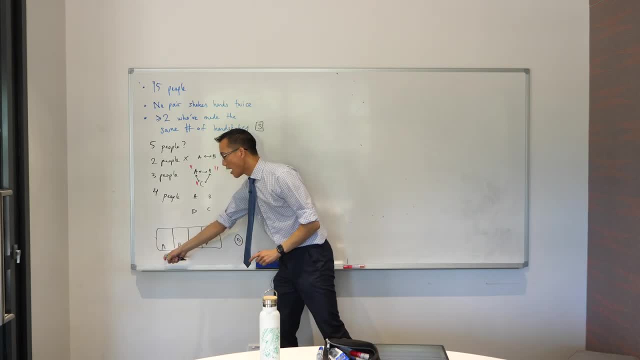 There are four available spots Even after they're all taken. the fifth one has to go somewhere, And there's a reason why there are only four pigeonholes possible in this situation. So let me pause right there and just have a think about the four people and what has 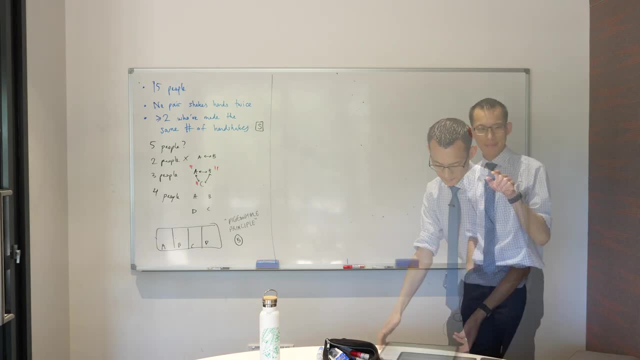 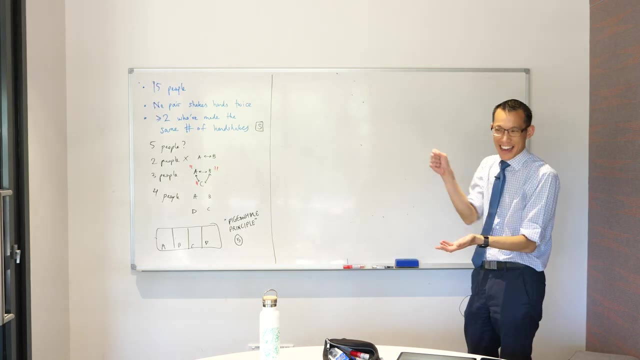 to happen. Just pause there and give you some time to think. I see you guys are still thinking. are you guys at a brick wall at the moment? That's totally okay. It just means I will not make you keep on beating your head against the brick wall. 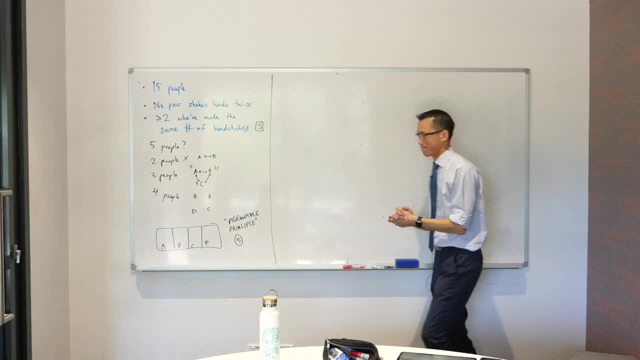 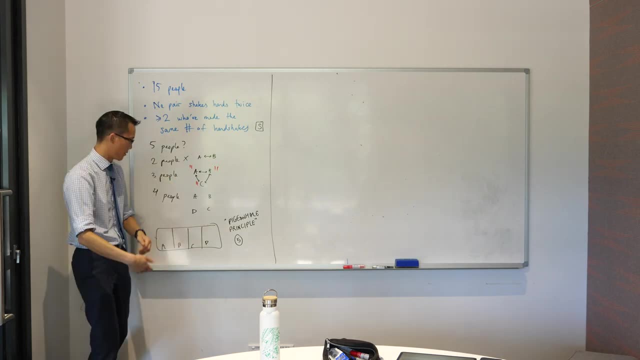 Yeah, Do you want me to jump in? Yeah, Okay, Here's where I'm, hopefully, because what I want to try and do is I could just read out the answer to you, but that's not helpful, right? I need to get you to that point. 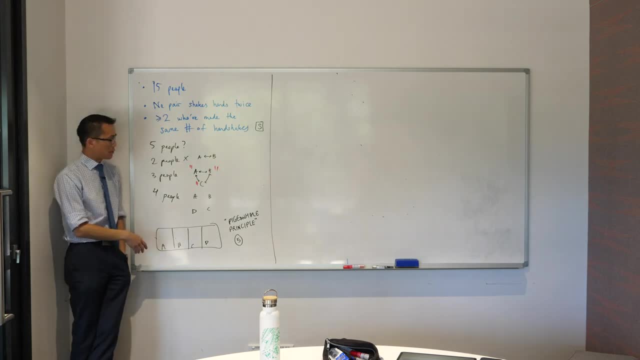 So I want you to return back to this idea of the pigeonhole principle, because at the moment, you've heard the pigeonhole principle but you're like: I don't know what the pigeons are, I don't know what the pigeonholes are, and that's the problem, right? 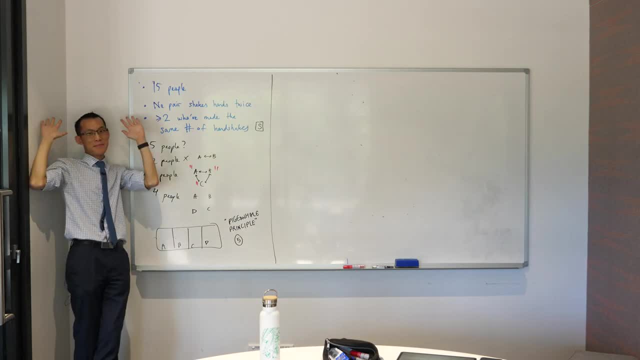 Once you know- sorry to keep on using the metaphor, but they named it, it's not me- Once you know what the pigeons are and once you know what the pigeonholes are. that's pretty much all there is to the problem. 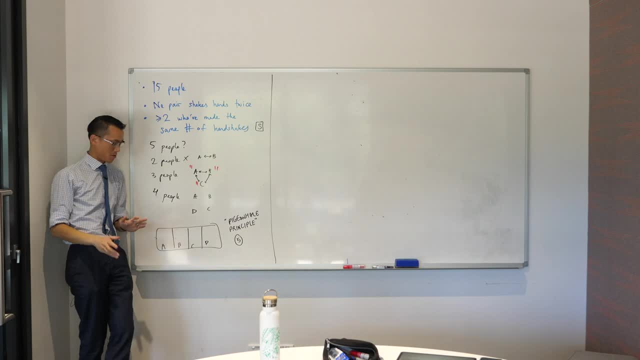 And then at the end you say by the pigeonhole principle, and then you walk away from the problem. So let me give you a suggestion about: well, I'll ask you the question. I think it might be not that difficult In this situation. what do you think the pigeons are? 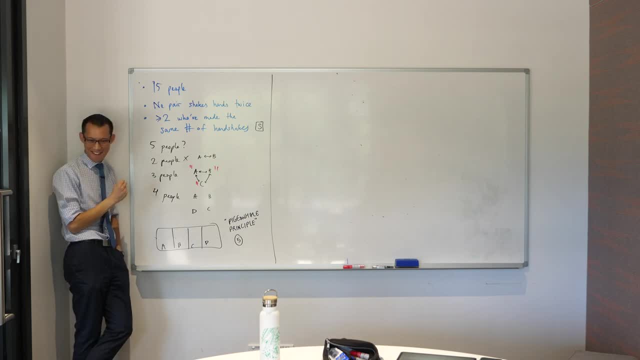 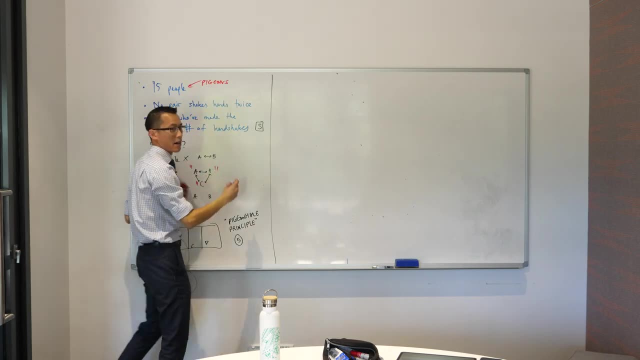 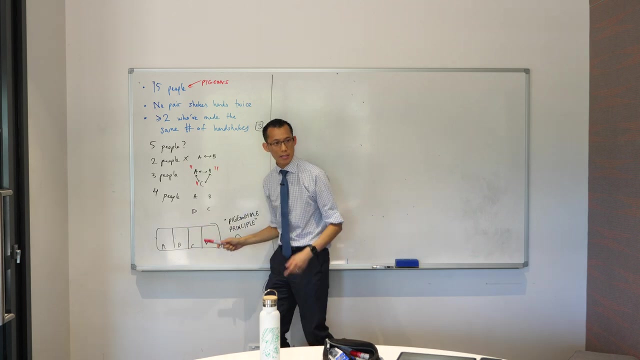 They're people, They're like the only objects that there are, right, So I'm going to suggest these are our pigeons. Now, the whole idea of how many pigeonholes are there is. each of the pigeons matches up to something. Now, in this question, what is the something we're trying to match them up to? 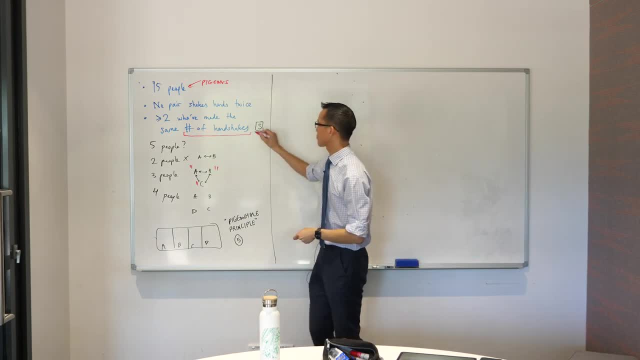 It's the number of handshakes. The number of handshakes is the pigeonholes, or you could do it vice versa. It's a symmetrical relationship, right? So I'm going to call these the pigeonholes. So, returning back to my illustration here- and thank goodness I'm not drawing any pigeons- 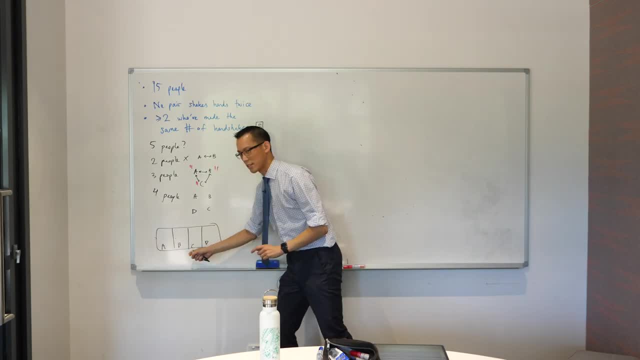 wonder if you're connecting it to this. yeah right, there are four available spots even after they're all taken. the fifth one has to go somewhere, and there's a reason why there are only four pigeonholes possible in the situation. so let me pause right there and just 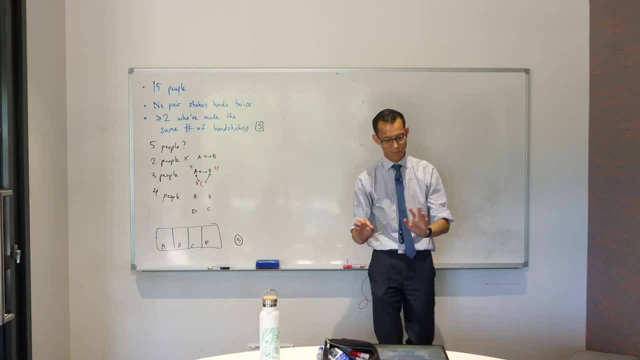 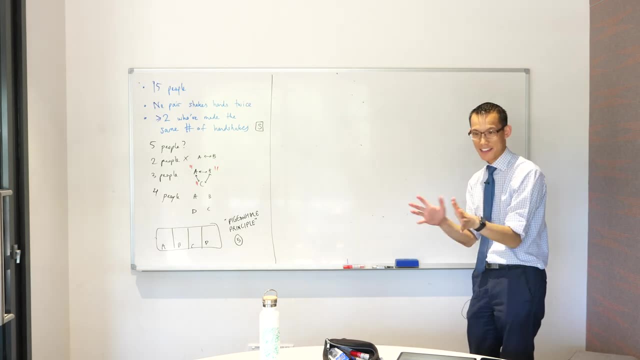 have a think about the four people and what has to happen. just pause there and give you some time to think. i see you guys are still thinking. are you guys at a brick wall at the moment? that's totally okay. it just means i will not make you keep on beating your head against the brick wall. 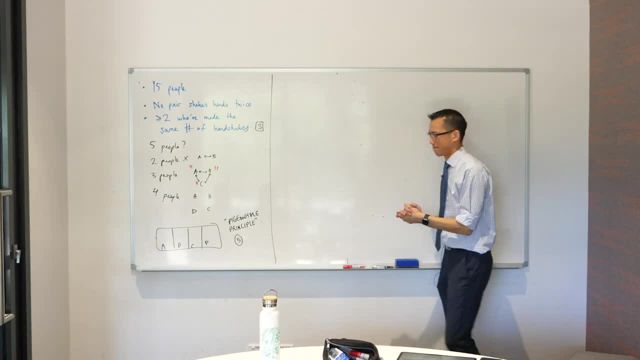 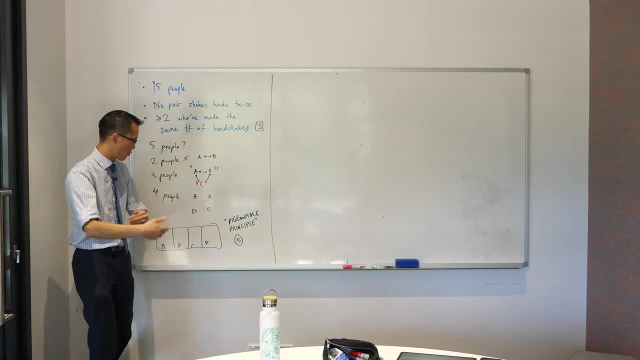 yeah, do you want me to jump in? yeah, okay, here's where i'm, hopefully, because what i want to try and do is like i could just read out the answer to you, but that's not helpful, right, i need to get you to that point. so i want you to return back to this idea of the pigeonhole principle. 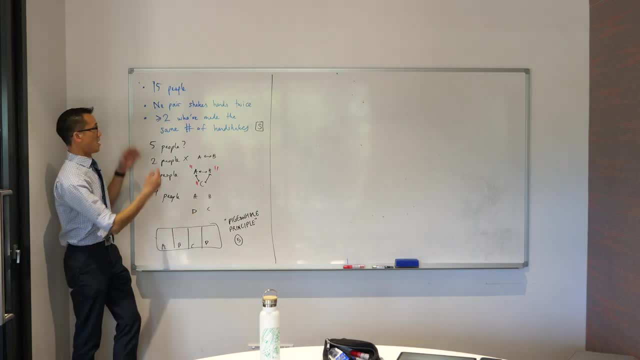 because at the moment, you've heard the pigeonhole principle but you're like: i don't know what the pigeons are and i don't know what the pigeonholes are, and that's the problem, right. once you know- sorry to keep on using the metaphor, but they named it, it's not me- once you know what the pigeons are, 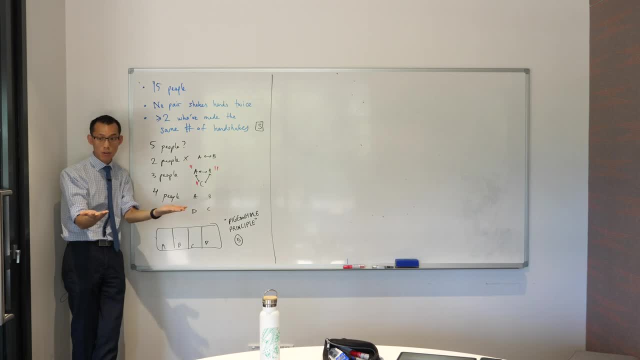 and once you know what the pigeonholes are, that's pretty much all there is to the problem. and then at the end you say: by the pigeonhole principle, and then you walk away from the problem. so let me give you a suggestion about: well, i'll ask you the question. i think it might be not that difficult. 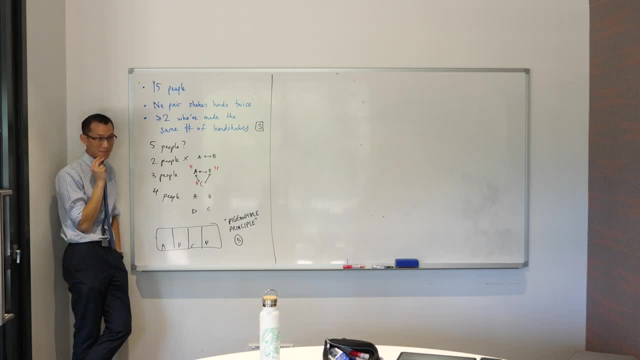 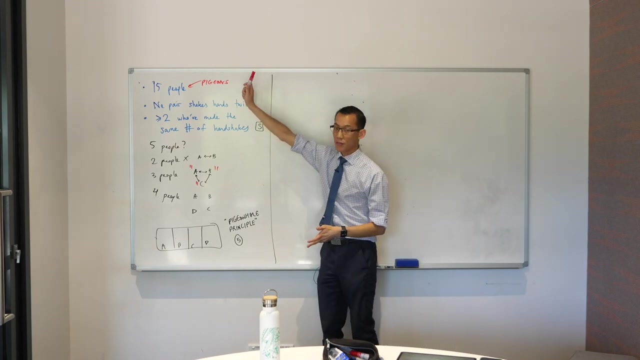 in this situation. what do you think the pigeons are? they're people. they're like the only objects that there are, right, so i'm going to suggest these are our pigeons. now, the whole idea of how many pigeonholes are there is each of the pigeons matches up to. 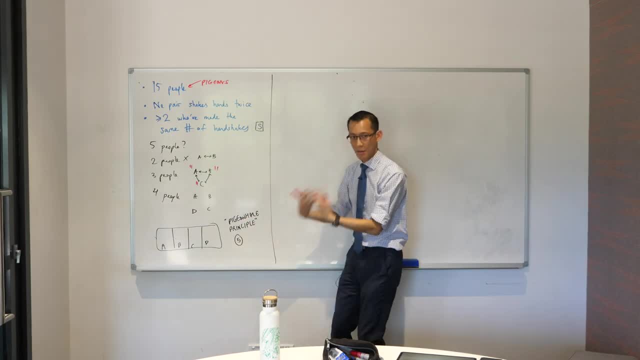 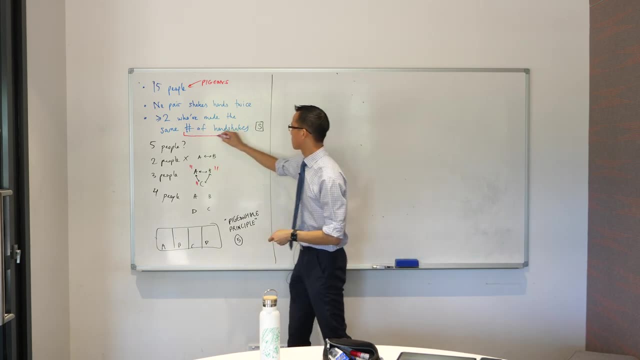 something now in this question. what is the something we're trying to match them up to? it's the number of handshakes. the number of handshakes is the pigeonholes, or you could do it vice versa. it's a symmetrical relationship, right? so i'm going to call these the pigeonholes. 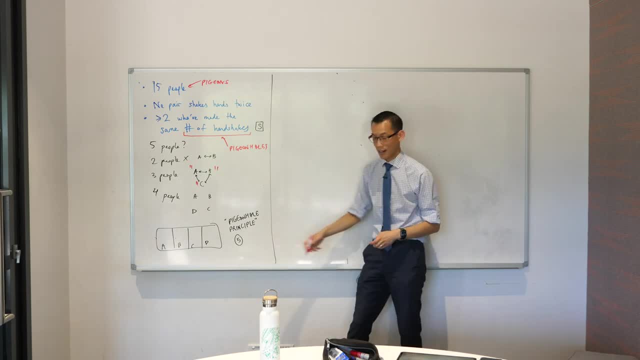 so, returning back to my illustration here- and um, thank goodness i'm not drawing any pigeons for you, because i can't- if i can prove that there are um fewer pigeonholes than pigeons, like, say, for example, four pigeonholes, five pigeons. right, that means that at least two of them are in the same. 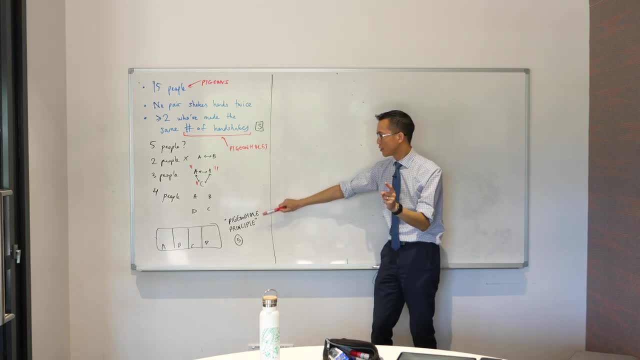 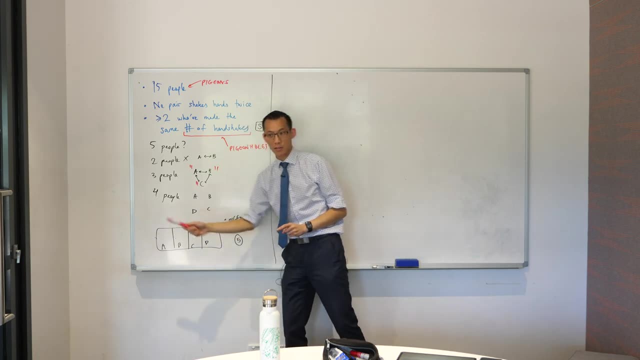 for you, because I can't. If I can prove that there are fewer pigeonholes than pigeons, like, say, for example, four pigeonholes, five pigeons, right, That means that at least two of them are in the same pigeonhole, which is the same do. 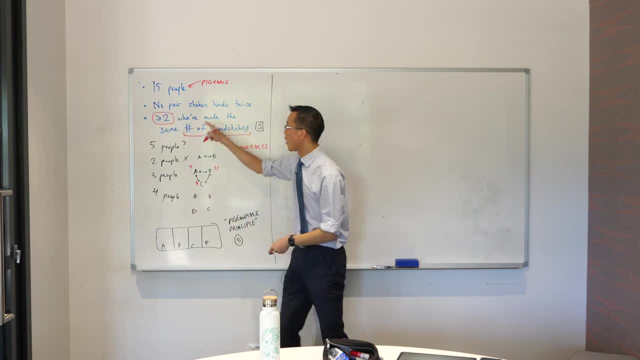 you see that phrase there- At least two of them who are in the same pigeonhole. That's me translating This language into this question. How are you with that? so far Is that okay, All right, Now let's just have a look back at our situation of four people. okay, because I think this: 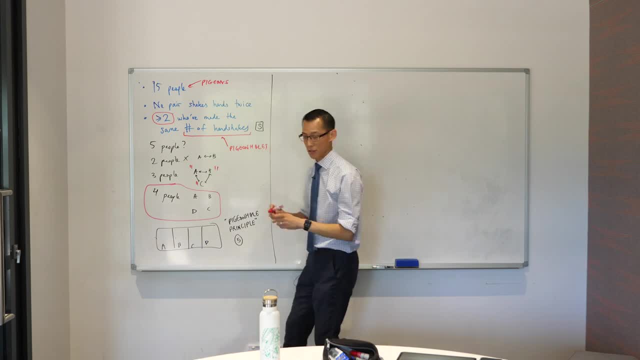 is now. it's starting to get complicated enough, but manageable. okay, The pigeonholes are the number of handshakes that are done right Now. given some of the information in the question, you can already tell me, for example, what's. 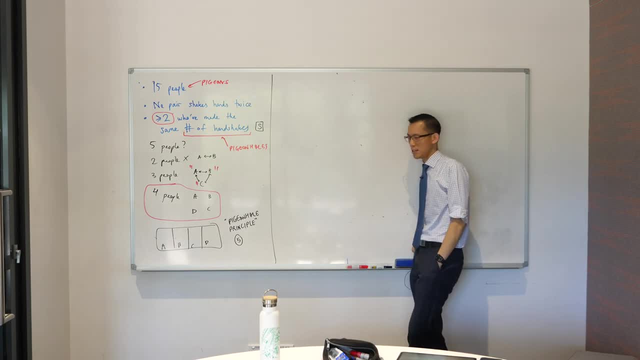 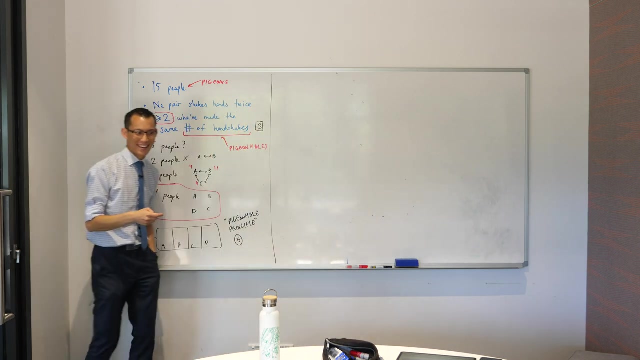 the maximum number of handshakes that happens In this situation of four people, like for A or B or C or D. what's the most handshakes any of them can do? Three. How did you get three? Have a think right. 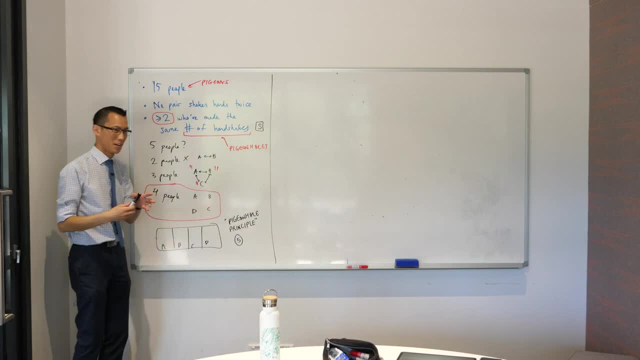 Like, this is the part that you guys need to do. If I tell you, then it's me doing the work, not you right? Why is it three? Well, at least two reasons. Number one, I mean you can have a look at the two previous examples that we just did. 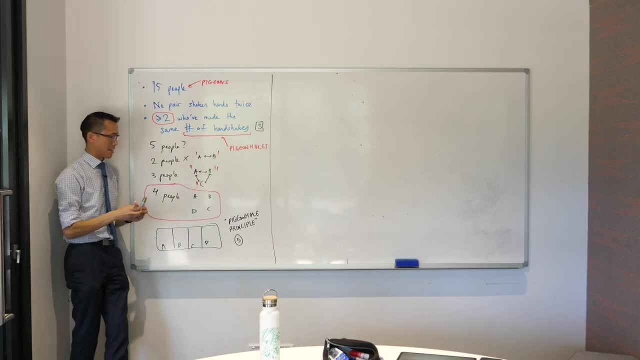 right, I didn't mark it in, but they both did one handshake and then they're done, finished. They both, they all, did two handshakes and then like, oh, I'm finished, right, Why is it that it has to be? I guess, if you call this N the maximum number of handshakes. 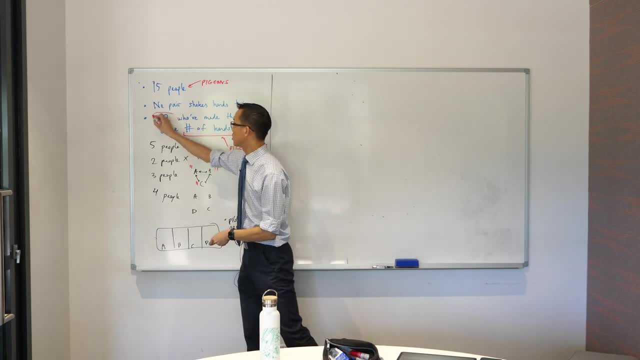 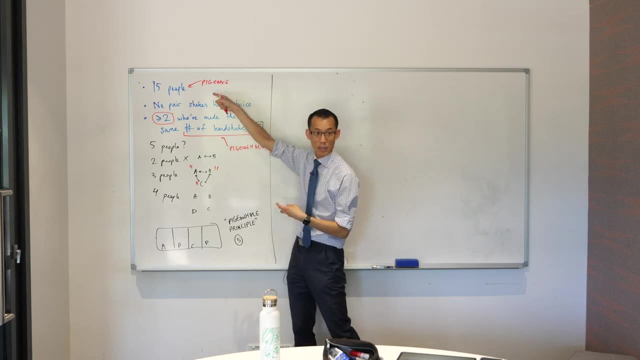 pigeonhole, which is the same. do you see? that's that phrase- there at least two of them who are in the same pigeonhole. that's me translating this language into this question. how are you with that so far? is that okay? all right, now let's just have a look back at our situation of four people. okay, because i think this: 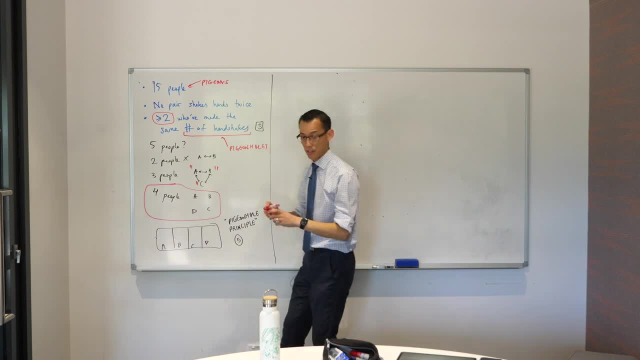 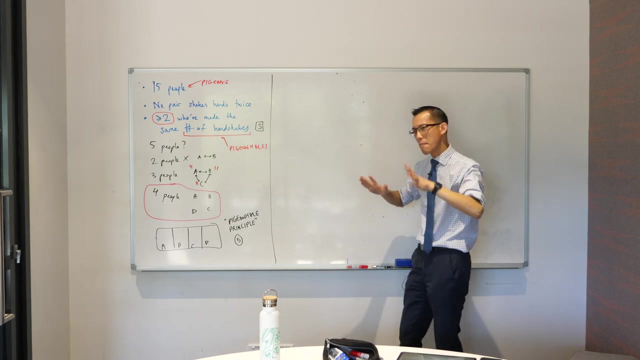 is um. now it's starting to get complicated enough, but manageable. okay, the pigeonholes are the number of handshakes that are done right now. given some of the information in the question, you can already tell me, for example, what's the maximum number of handshakes that happens in this situation. 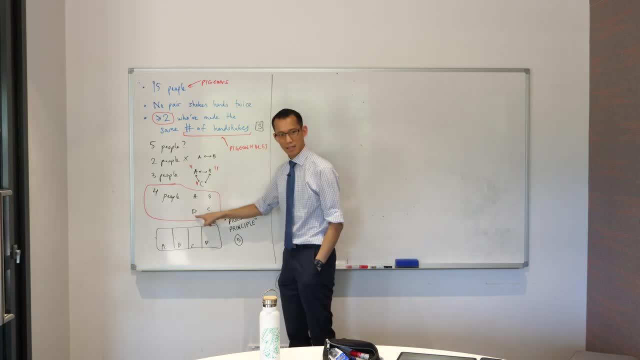 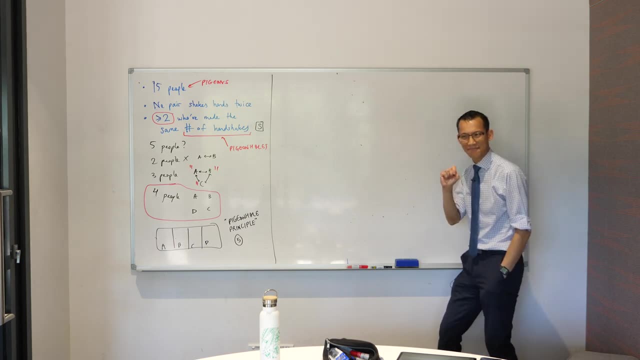 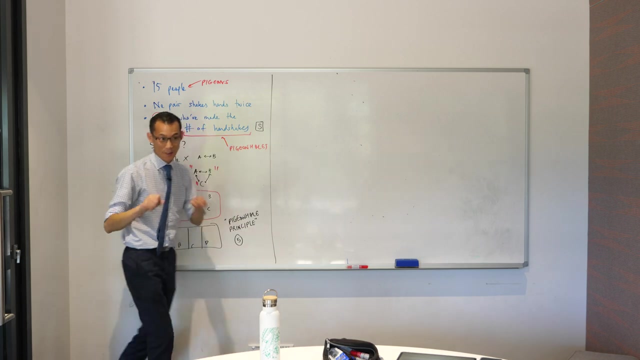 of four people, like for a or b or c or d, what's the most handshakes? any of them can do three. how did you get three? have a think right like: this is the part that you guys need to do. if i tell you, then it's me doing the work, not you right? why is it three? well, at least two reasons. number one: 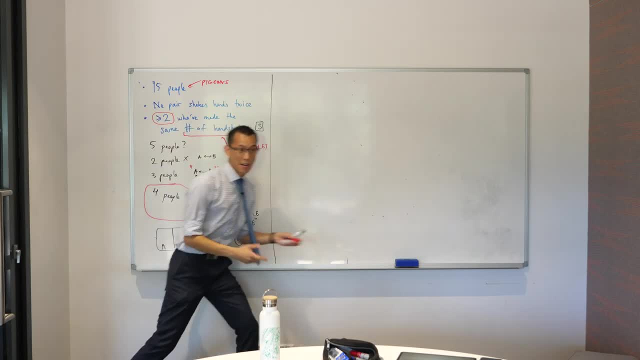 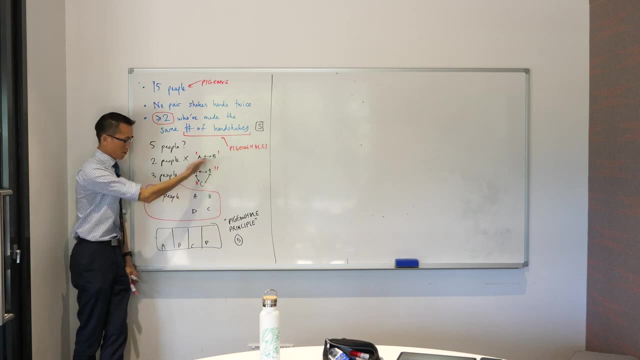 i mean you can have a look at the two previous examples that we just did right, you can follow the pattern. uh, i didn't mark it in, but they both did one handshake and then they're done, finished. they both, they all did two handshakes and then like, oh, i'm finished, right. 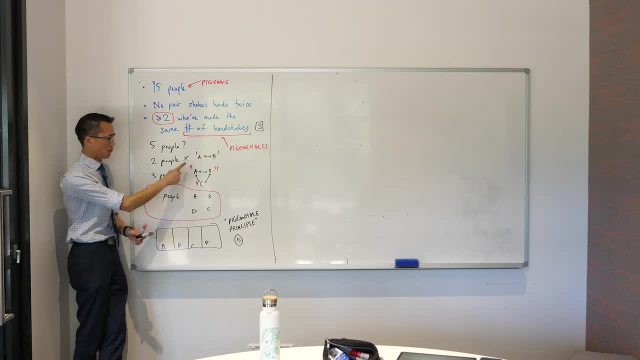 why is it that it has to be? i guess, if you call this n, the maximum number of handshakes has to be n minus one. you can't shake hands with yourself. so there's four people here, but i'm like i can't. i can't do that, so the only options are the other three people. 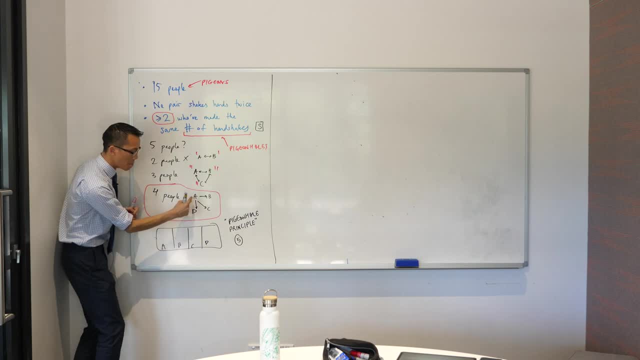 yes, so because it's the other people minus you, you're the one right, so that's why you end up with this um n minus one. okay, does that make sense so far? 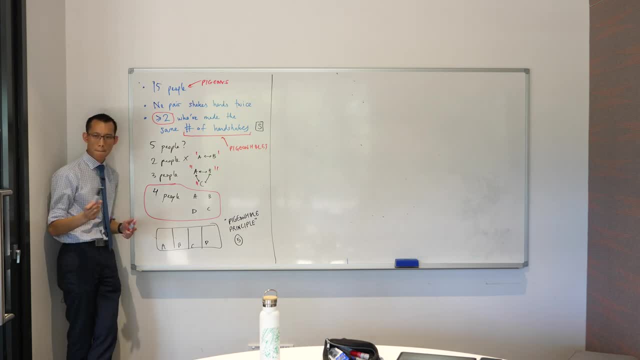 has to be N minus one. You can't shake hands with yourself. You can't shake hands with yourself. So there's four people here, but I'm like I can't. I can't do that, So the only options are the other three. 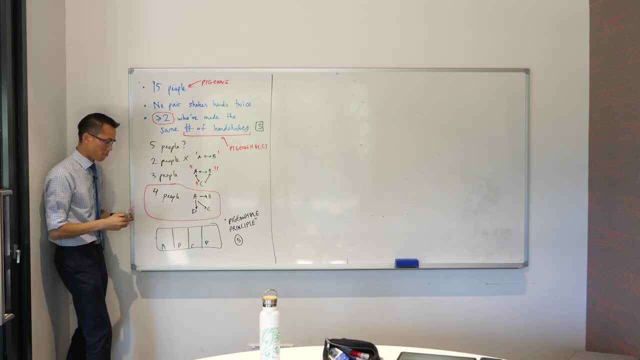 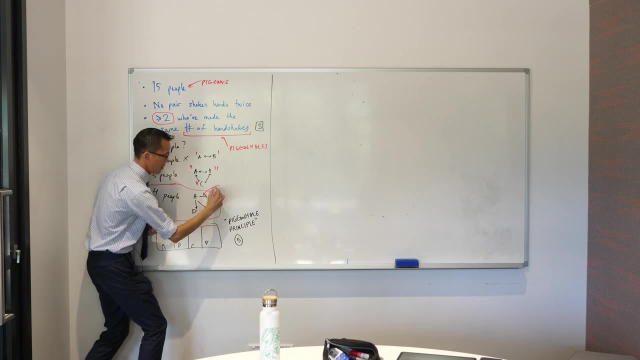 Three people. yes, So because it's the other people minus you, you're the one right. So that's why you end up with this N minus one. Okay, Does that make sense so far?